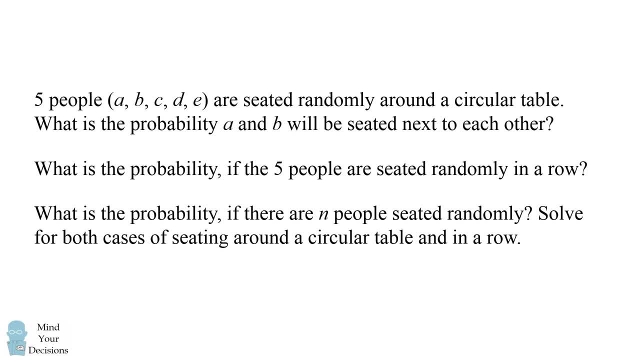 What is the probability if there are N people seated randomly? Solve for both cases of seating around a circular table and in a row. This problem has been asked to programmers and during other technical jobs as an interview question. Can you figure it out? Give this problem a try and, when you're ready, keep watching the video for the solution. 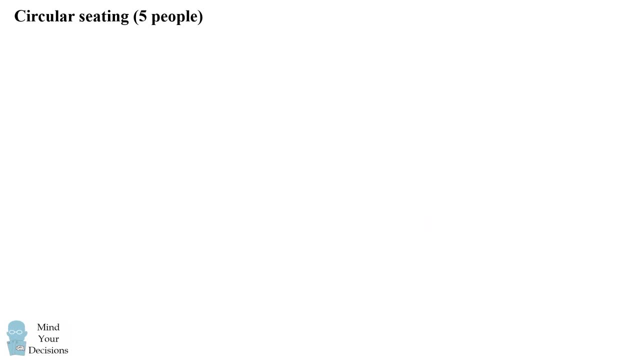 We'll first consider seating around a circular table with five people. There are a couple of ways we'll solve this. The first method is we'll consider equally likely seats. We have a circular table with five different seats. Person A will be in some seat. 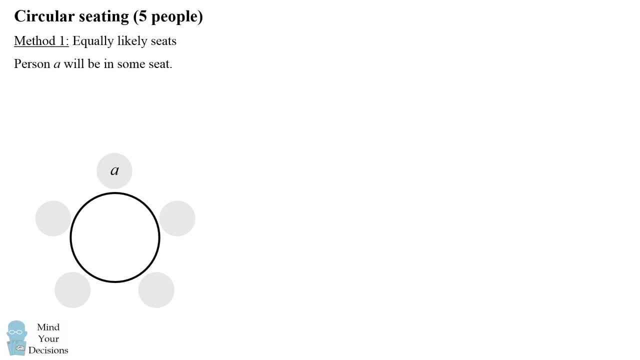 Without loss of generality, we can make it the seat at the top of the diagram. Person B can be in any of the four remaining seats and it's equally likely that B will be in any of these seats. Of these seats, exactly two of them will be adjacent to A. 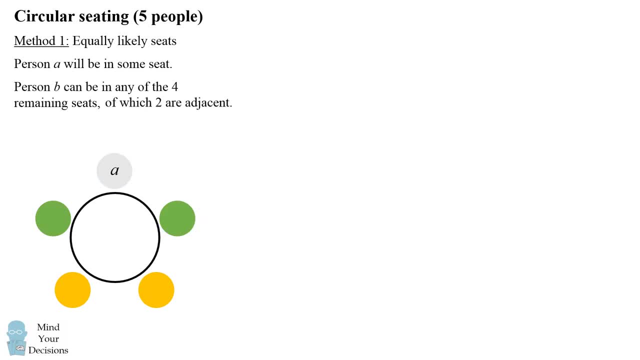 Therefore, the probability that A and B will be seated adjacent is two divided by four, which equals one half, and that's fifty percent. There's another way you could solve the problem: by counting pairs of seats. When there are five seats, there are five. choose two, which equals ten pairs of seats. 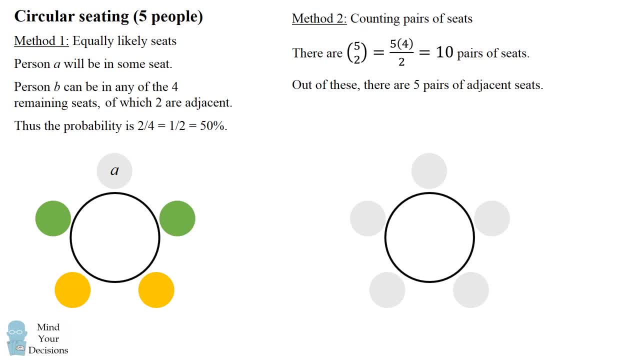 Out of these, there are five pairs that are adjacent. Each seat can be paired adjacently to the one that's right next to it, going clockwise. Therefore, the probability that A and B will be adjacent will be five divided by ten, which also equals one half, and that's also fifty percent. 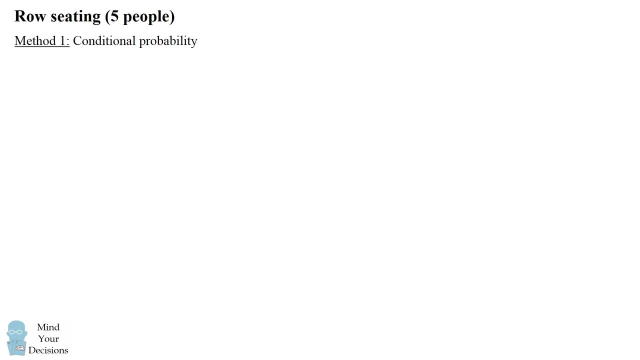 Let's now solve the problem of seating in a row. One way to solve this is to use conditional probability. There are two different ways that A could be seated. Person A could be in the first or the last seat. These are two out of five possible seats. 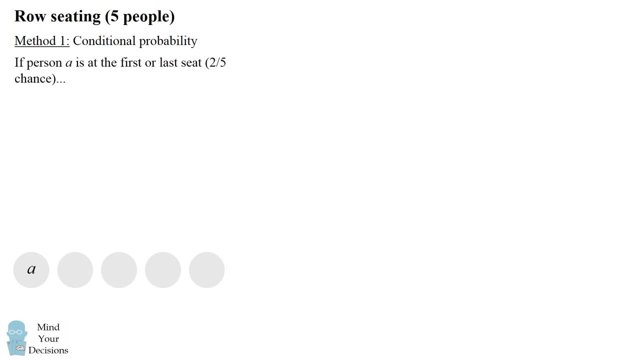 So if person A is in the first seat, for example, then person B will be adjacent for exactly one of the four remaining seats. Similarly, if person A is at the end seat, person B has to be right next to it. That's one out of the four remaining seats. 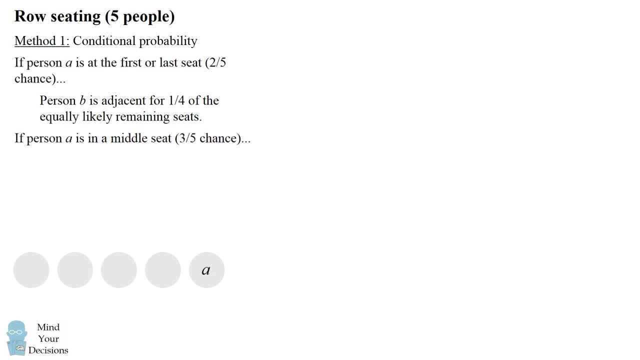 Now there's another case that person A could be in the first or the last seat, and that's one out of the four remaining seats. So in this five-person case there are three middle seats. In any of these seats person B can be adjacent to be either on the left side or the right side. 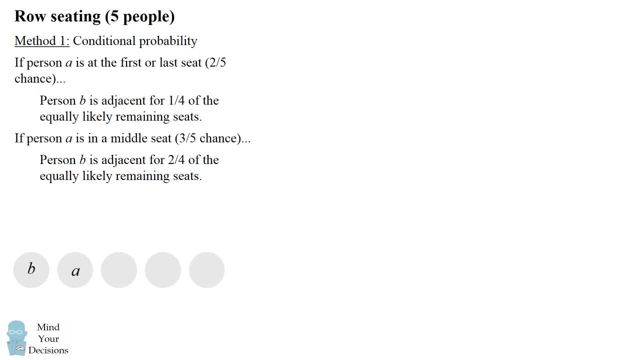 There are two places that person B could be and could be adjacent. So if we put these cases together, the probability is two over five times one over four, plus three over five times two over four, and that simplifies to be two-fifths, which is forty percent. 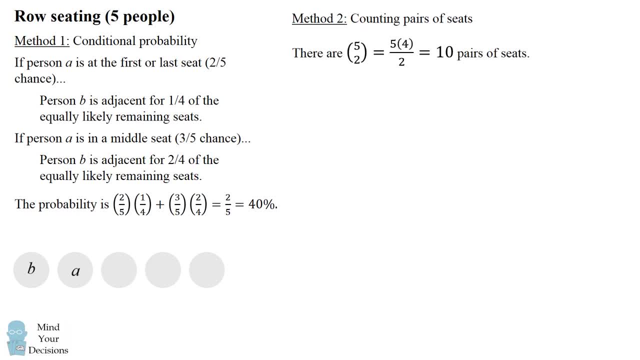 Another way is that we could count the pairs of seats. There are five. choose two, which is ten pairs of seats. Now, how many of these are adjacent? Well, there are four pairs of adjacent seats because the first, the second, the third and the fourth seats could be paired with the seat after it. 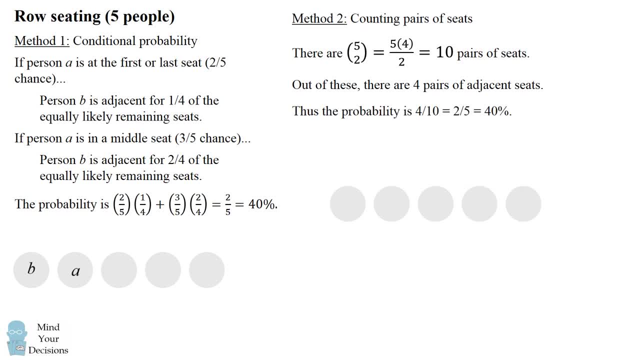 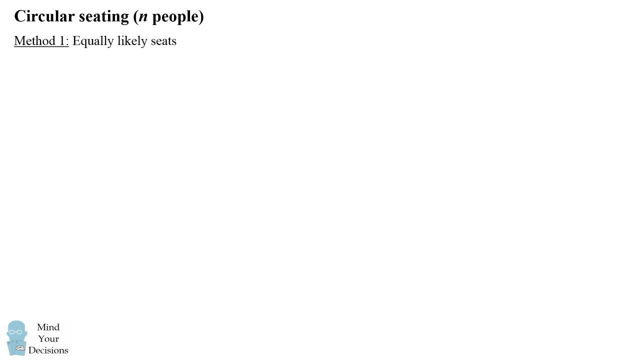 Therefore, there are four out of ten possibilities, which also equals forty percent. Now let's generalize for n people. We could solve these in the same ways. Let's consider the method of equally likely seats. Person A will be at some seat. 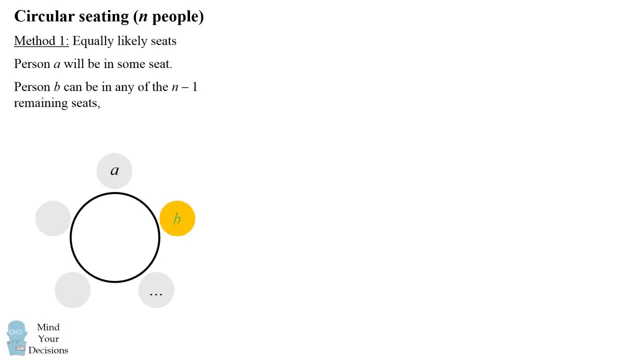 and now person B can be any of the n minus one remaining seats, and it's equally likely that B will be at any of these n minus one remaining seats. Out of them, exactly two will be adjacent: the seat to the left and the seat to the right, of person A. 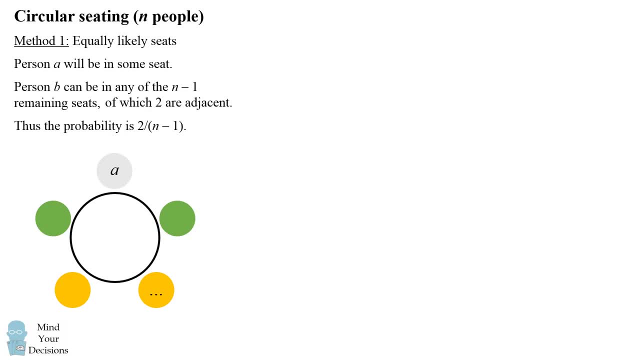 Therefore there will be exactly two divided by n minus one possible ways that a and B could be next to each other. So the probability is two over n minus one. We can also do the same thing by counting the pairs of seats. There are n. choose two, which equals n times n minus one over two pairs of seats. 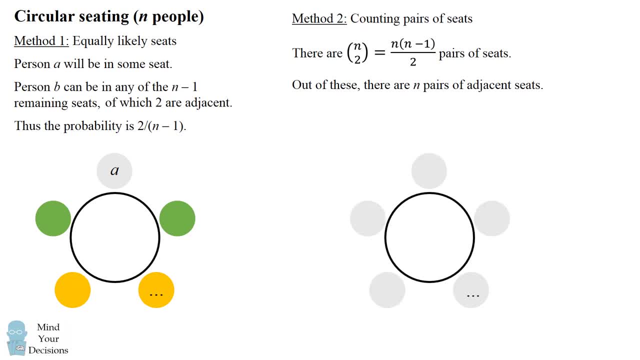 Out of these, there are n pairs of adjacent seats, And we start from the top of the seat diagram and go clockwise. each seat can be paired with the one right after it. We end up counting n different pairs of adjacent seats. So if we take n divided by n, choose 2, this also simplifies. 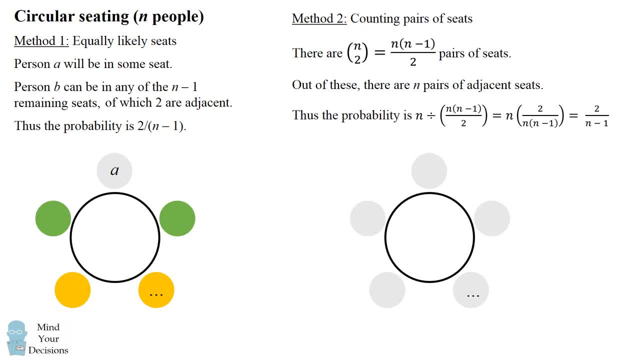 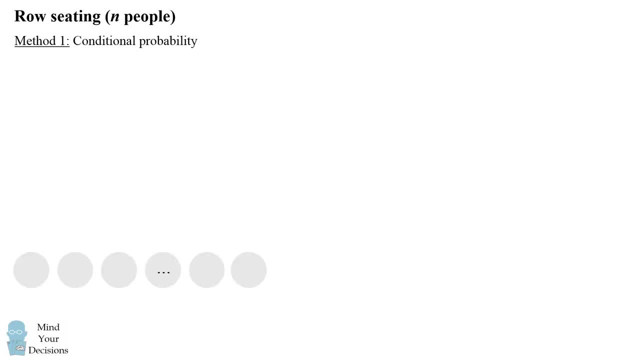 to be 2 divided by n minus 1.. Let's now solve the case of seating in a row where you have n people. We can again solve it by conditional probability. The one case is that a is either in the first seat or the last seat. 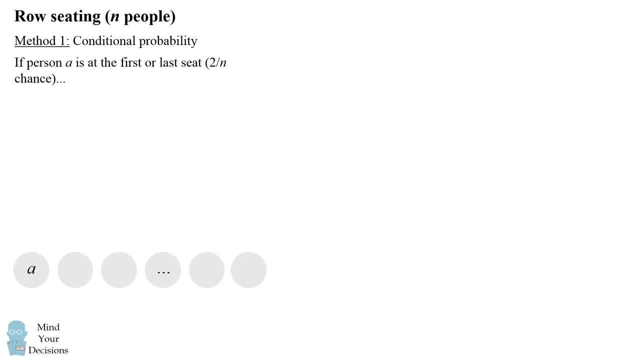 So these will be two out of the n possible seats. So in the first seat person b could be adjacent. for only one out of the n minus 1 remaining seats It would have to be just right after, Or if a was at the very end, b would have to be just before. 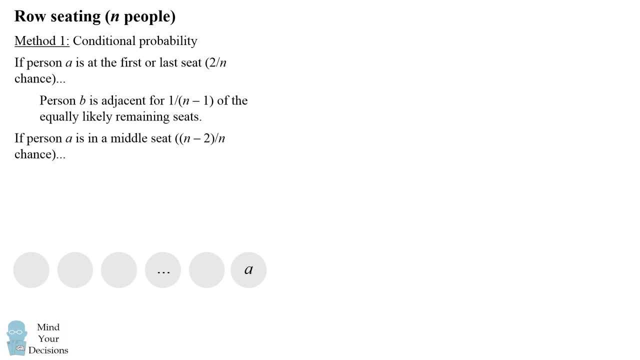 Now there's also the other case that a could be in a middle seat. There are n minus 2 out of a total n middle seats. In any of these middle seats, b could either be on the left side or the right side. So there will be two out of the n minus 1 possible ways that b could be adjacent. 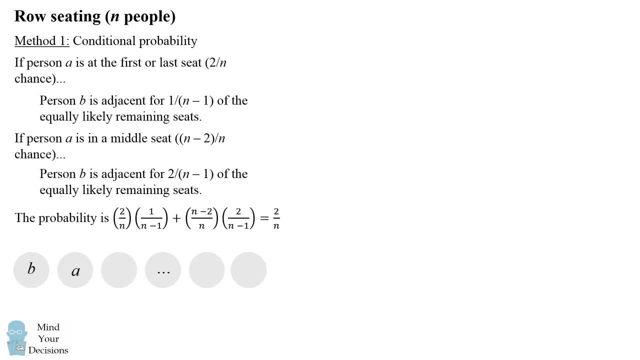 If we combine these cases, we end up with the following equation: 2 over n times 1 over n minus 1 plus n minus 2 over n times 2 over n minus 1.. If you work through the algebra, this simplifies to be 2 over n, and that's. 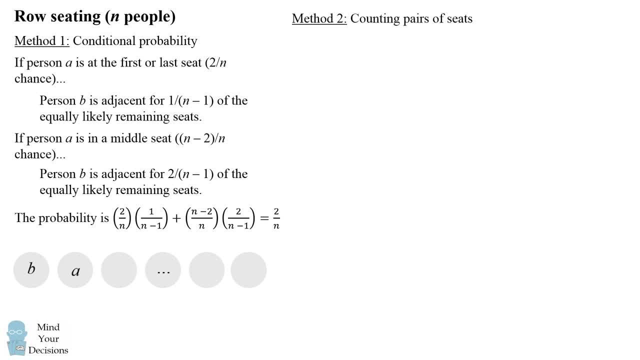 the probability. We could also do the same thing by counting pairs of seats. There are n. choose 2 pairs of seats. And now how many adjacent seats are there? Well, they're n minus 1.. Each seat can be paired with the seat to its right. 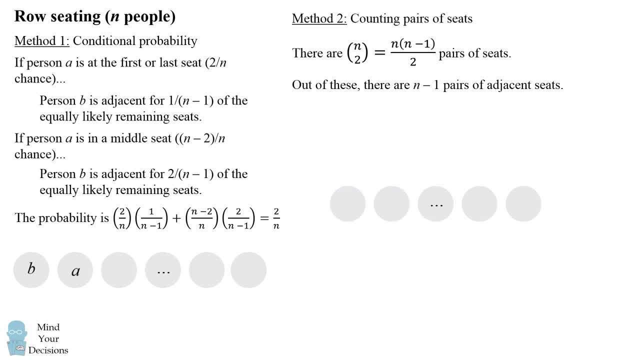 So, starting from the first seat on the left, we can count all the way up to n minus 1.. That very last seat has no seat to its right. Therefore, we take n minus 1 and divide it by n choose 2.. 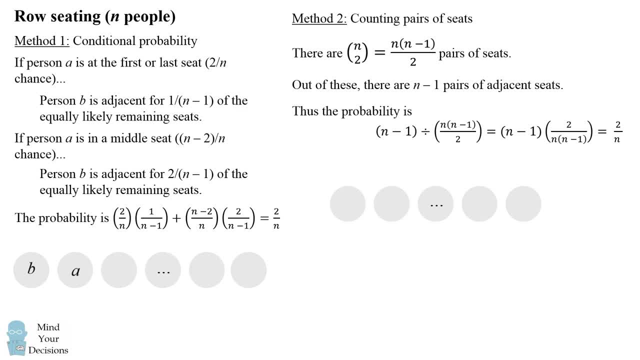 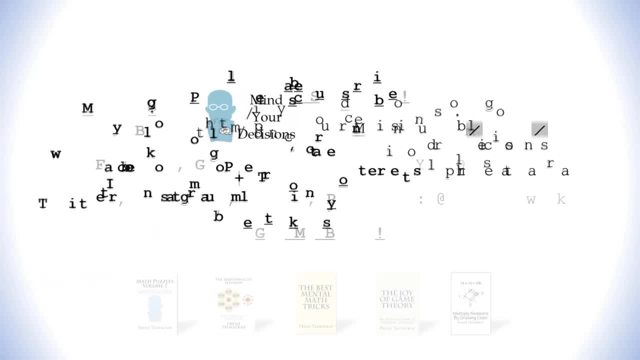 And that also simplifies to be 2 over n. Did you figure out these problems? Thanks for watching this video. Please subscribe to my channel. I make videos on math. You can catch me on my blog Mind Your Decisions, which you can follow on Facebook. 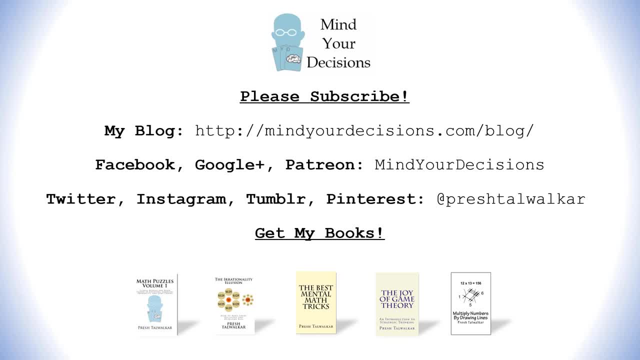 Google Plus and Patreon. You can catch me on social media at Presh Talwalkar And, if you like this video, please check out my books. There are links in the video description.